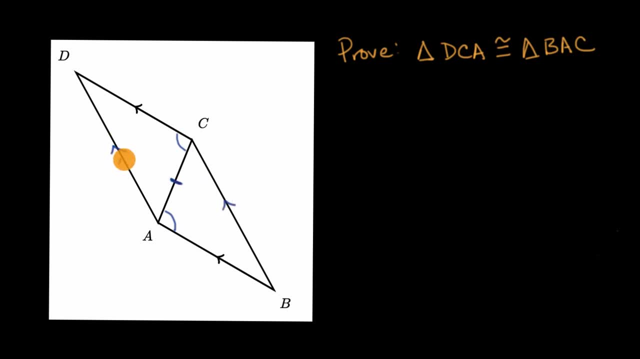 thinking that this is parallel to that because it looks parallel. but you can't make that assumption just based on how it looks. If you did know that, then you would be able to make some other assumptions about some other angles here and maybe prove congruency. 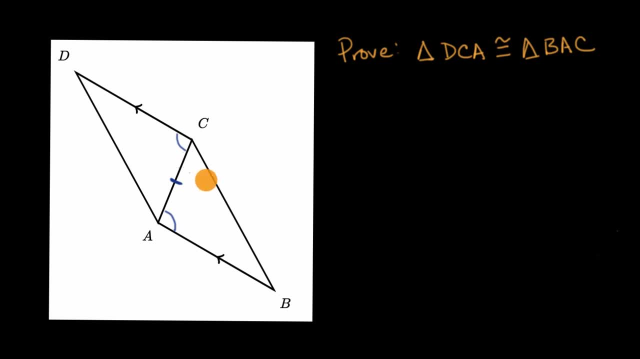 But it turns out, given the information that we have, we can't just assume that because something looks parallel or because something looks congruent that they are, And so, based on just the information given, we actually can't prove congruency. Now let me ask you a slightly different question. 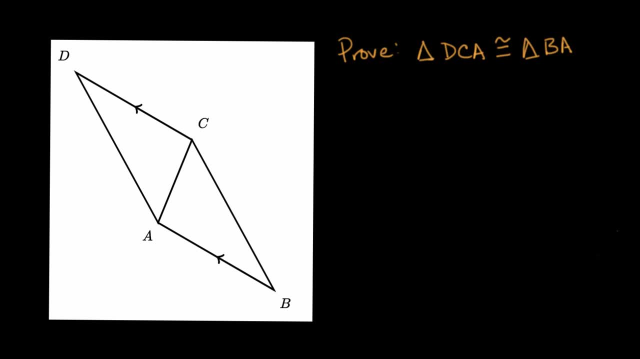 Let's say that we did give you a little bit more information. Let's say, we told you that the measure of this angle right over here is 31 degrees and the measure of this angle right over here is 31 degrees. Can you know that? 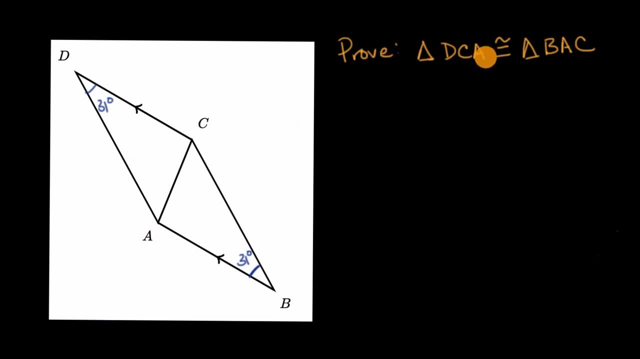 Can you now prove that triangle DCA is congruent to triangle BAC? So let's see what we can deduce now. Well, we know that AC is in both triangles, so it's going to be congruent to itself, And let me write that down. 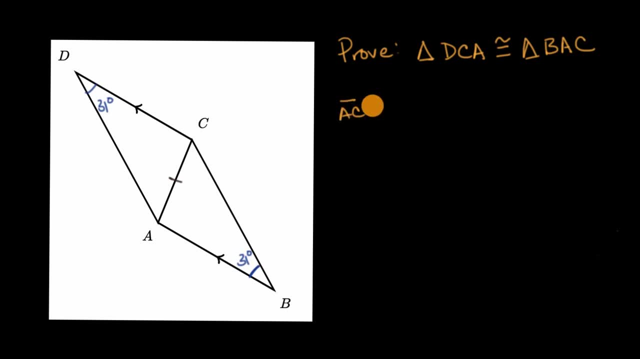 We know that segment AC is congruent to segment AC. It sits in both triangles and this is by reflexivity, Which is a fancy way of saying that something is going to be congruent to itself. Now we also see that AB is parallel to DC, just like before. 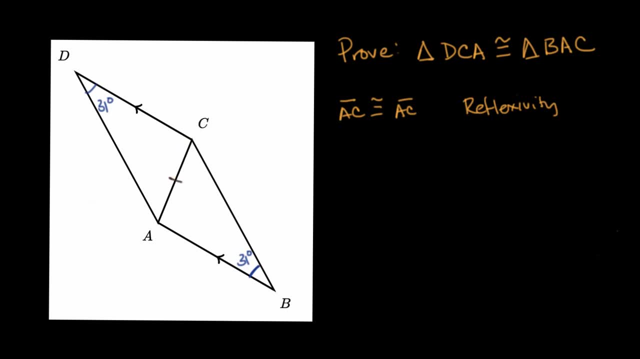 and AC can be viewed as part of a transversal, So we can deduce that angle CAB. let me write this down. Actually, let me do it in a different color. We can deduce that angle CAB is congruent to angle AC. 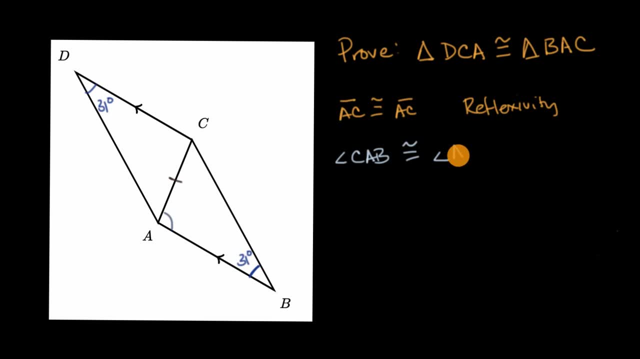 This angle is known as angle ACD, angle ACD because they are alternate, alternate interior, interior angles where a transversal intersects two parallel lines. So, just to be clear, this angle, which is CAB, is congruent to this angle. 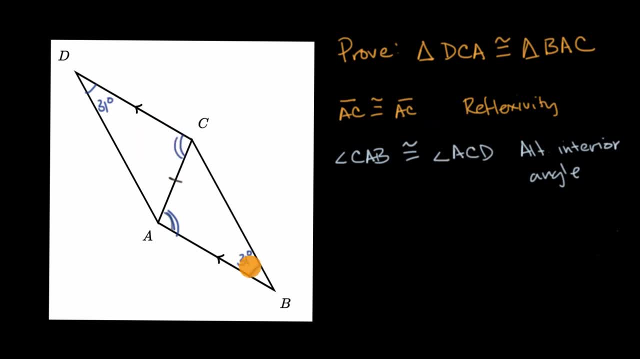 which is ACD. And so now we have two angles and a side, two angles and a side that are congruent. So we can now deduce by angle-angle-side postulate that the triangles are indeed congruent. So we now know that triangle DCA is indeed congruent. 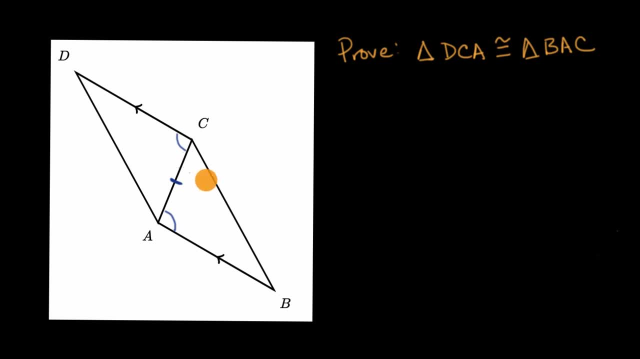 But it turns out, given the information that we have, we can't just assume that because something looks parallel or because something looks congruent that they are, And so, based on just the information given, we actually can't prove congruency. Now let me ask you a slightly different question. 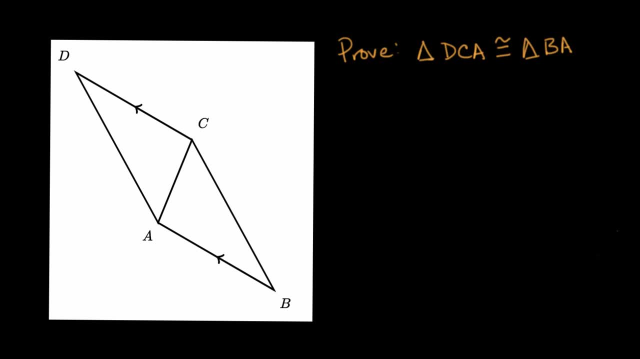 Let's say that we did give you a little bit more information. Let's say, we told you that the measure of this angle right over here is 31 degrees and the measure of this angle right over here is 31 degrees. Can you know that? 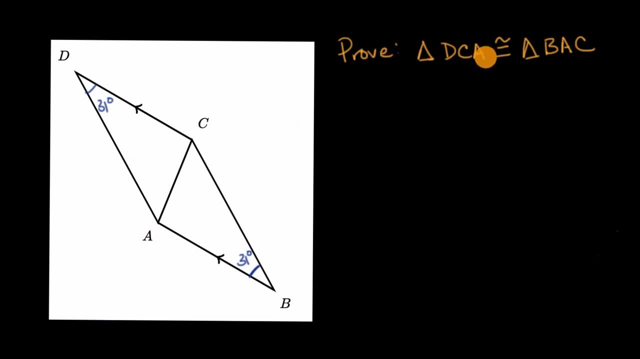 Can you now prove that triangle DCA is congruent to triangle BAC? So let's see what we can deduce now. Well, we know that AC is in both triangles, so it's going to be congruent to itself, And let me write that down. 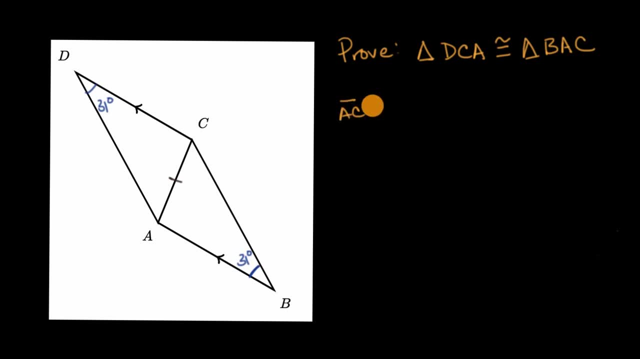 We know that segment AC is congruent to segment AC. It sits in both triangles and this is by reflexivity, Which is a fancy way of saying that something is going to be congruent to itself. Now we also see that AB is parallel to DC, just like before. 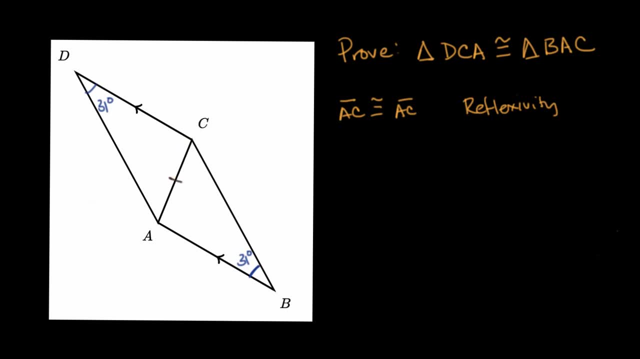 and AC can be viewed as part of a transversal, So we can deduce that angle CAB. let me write this down. Actually, let me do it in a different color. We can deduce that angle CAB is congruent to angle AC. 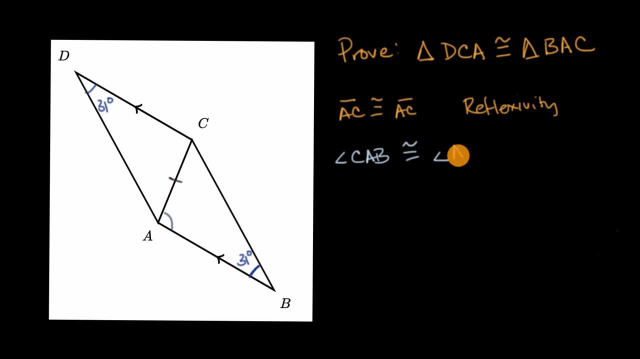 So this angle, so angle ACD, angle ACD because they are alternate, alternate interior, interior angles where a transversal intersects two parallel lines. So, just to be clear, this angle, which is CAB, is congruent to this angle. 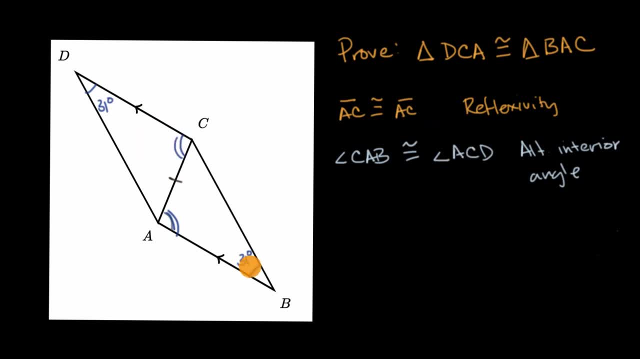 which is ACD. And so now we have two angles and a side, two angles and a side that are congruent. So we can now deduce by angle-angle-side postulate that the triangles are indeed congruent. So we now know that triangle DCA is indeed congruent.